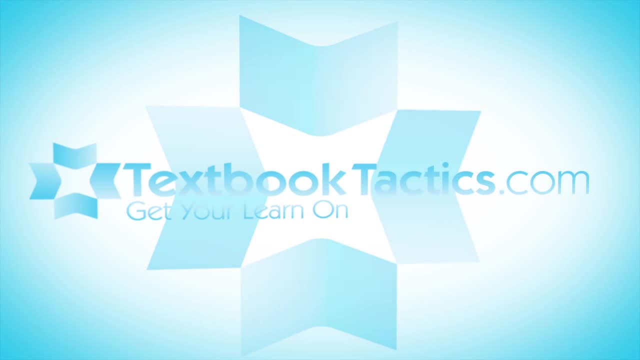 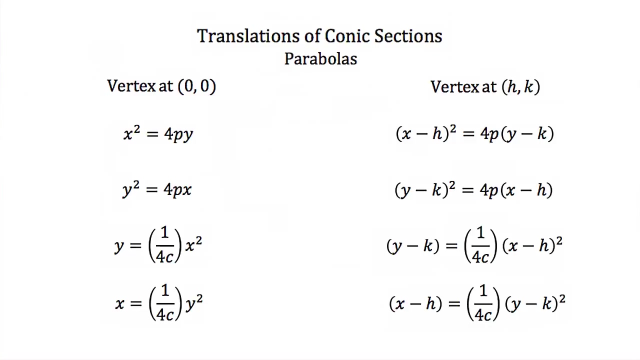 This is a tutorial on translations of conic sections. The first type of conic section that we're going to talk about translating is the parabola. Now you should know a standard form equation for a parabola that has its vertex at the origin. These standard form equations usually 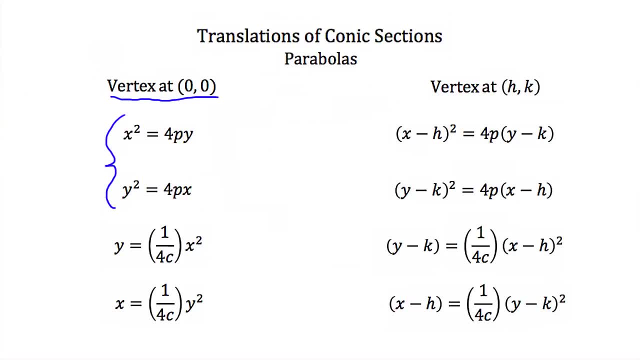 look in one of two ways. Either way, they have a value of p or c, or a value that tells us the distance between our vertex and our focus, or the distance between our vertex and our directrix. Well, what if our parabola doesn't have its vertex at the origin? What if it's got it at the point? 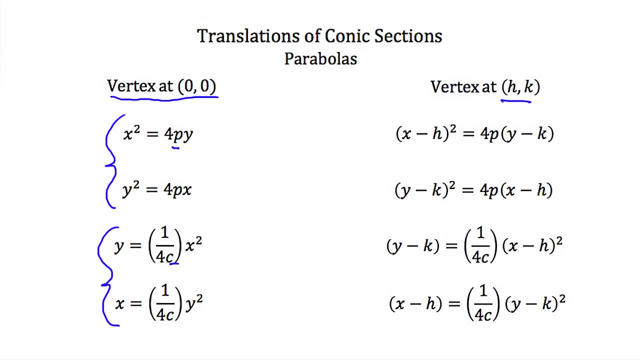 hk. If this point was the point 3,4, that would mean that h is 3 and k is 4.. So if our parabola has its vertex at hk, then we have a slightly different standard equation. But there's a pattern to be seen here As we translate our parabola, instead of having an 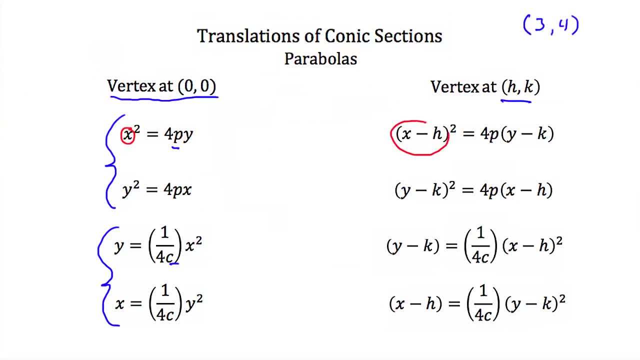 x in our equation, we have an x minus h. Instead of having a y in our equation, we have a y minus k. Now, if this is a y squared, then this is a y minus k squared. And don't forget that if you had y minus k, 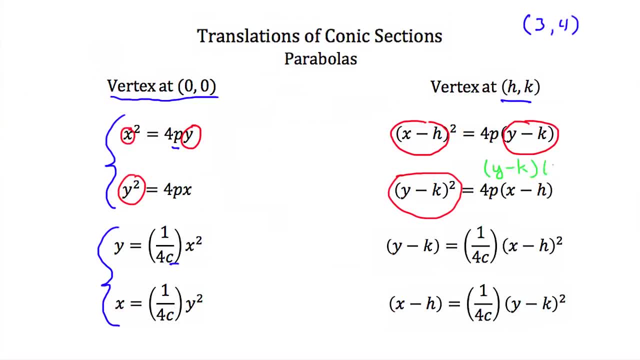 squared, that's the same as y minus k times y minus k, And if you have 4p times x, then you still have 4p times x minus h in parentheses. But what's important to notice is that in all of these new translated equations the value of p is 4p times x minus h. So if you have 4p times x minus h, you 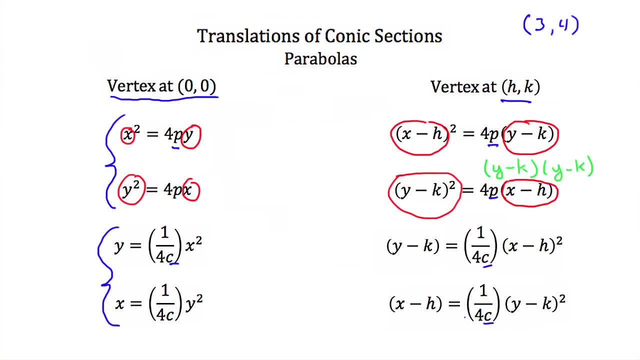 have 4p times x minus h. So the value of p and the value of c, depending on what you're taught in your textbook. that value hasn't changed The value of p or c. this determines the shape of our parabola. Changing the vertex only changes the location of our parabola, But again, the shape of 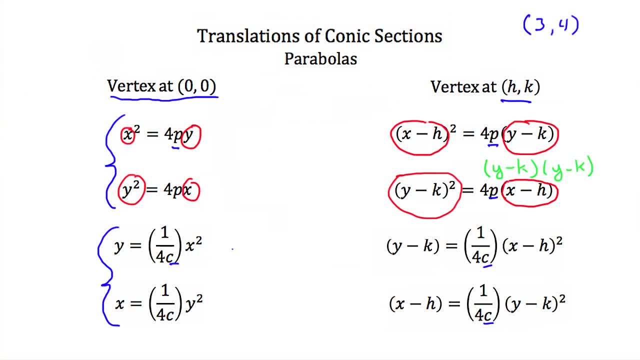 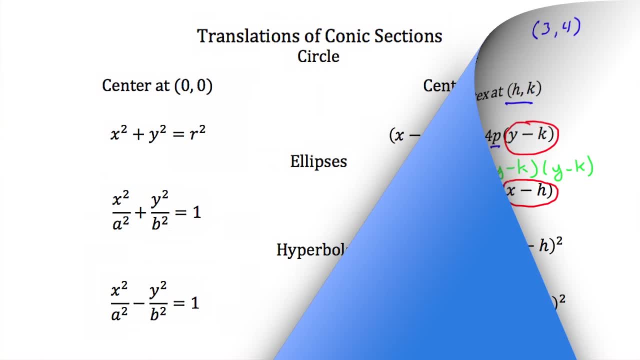 it is still determined by the value of p or c. So even though we've moved our parabola, that value doesn't change, because it's the same parabola. The same thing works for circles, ellipses and hyperbolas. 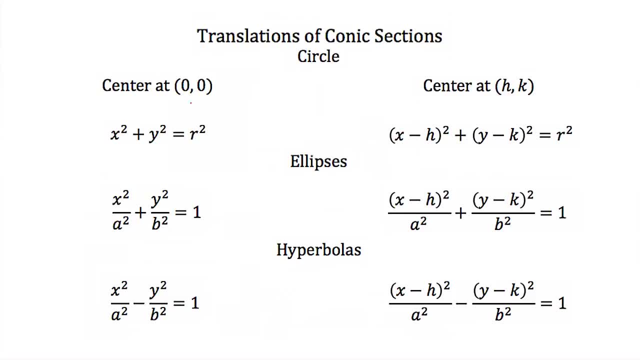 If you're going to move the center of your circle, ellipse or hyperbola from 0, 0 to h k, the only thing that changes is where you have an x, you have an x minus h. Wherever you have a y, you have a y minus k. 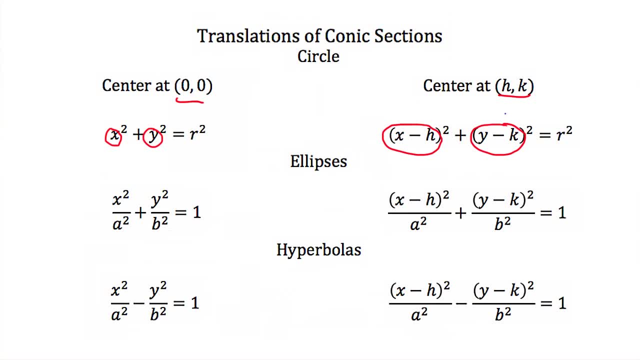 But again, notice, with a circle, even though we have a y, we have a y minus k. So even though we've translated it or moved it, our radius value doesn't change because the size of our circle hasn't changed. Even though we've moved our ellipse, our a and b values stay the. 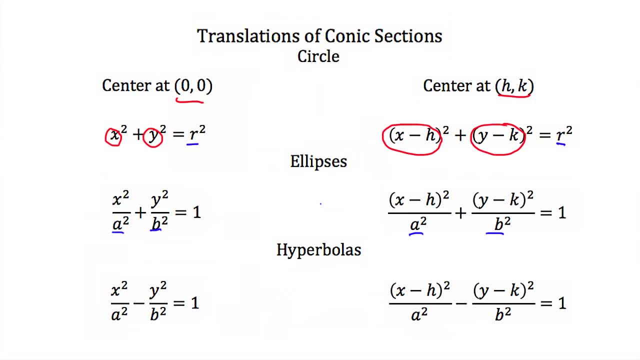 same, because we're not changing our major or minor axis lengths. we're just moving those axes. Same thing with a hyperbola: Our a and b values don't change, even though we have an x minus h instead of an x and a y minus k instead of a y. 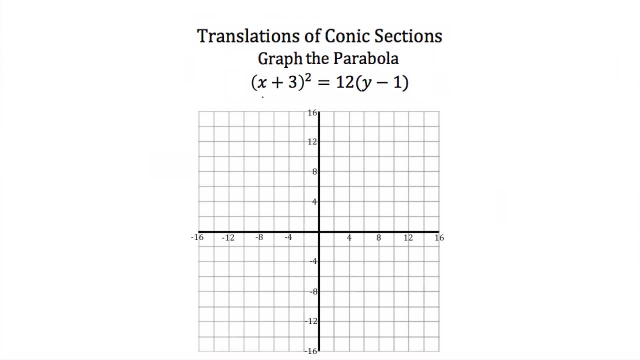 So now let's try taking what we've learned and let's graph the parabola: x plus 3, squared is equal to 12 times y minus 1.. This equation is in the standard form of x minus h, squared is equal to 4p times y minus k. 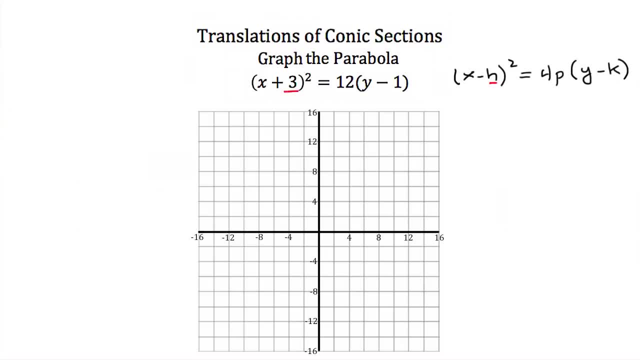 Right away we can tell that our h is negative 3, and our k is a positive 1.. So immediately we know that our vertex is the point negative 3, 1.. And I can plot that point. It would be right here Now, just like graphing a parabola with its vertex at the origin. 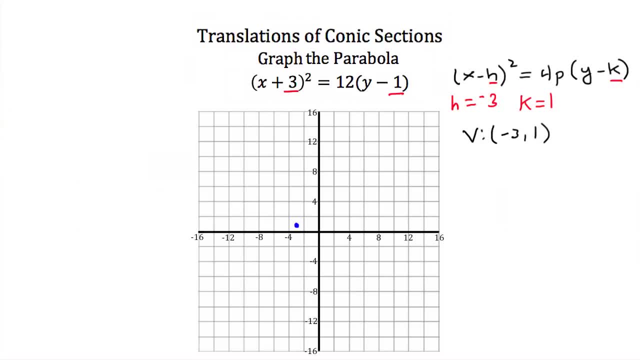 I go and I look at my p or my c value, which in this case I have a 4p- is equal to 12, so p, or, if you're familiar with c, that would be equal to 3.. This value is positive and we're having our x variable being squared. 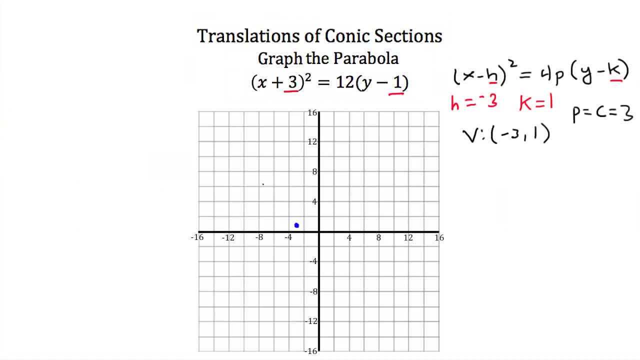 So, since our x variable is being squared, this parabola is going to open in either the positive or negative y directions. and because our p or c value is positive, that means it's going to open in the positive y direction. So our 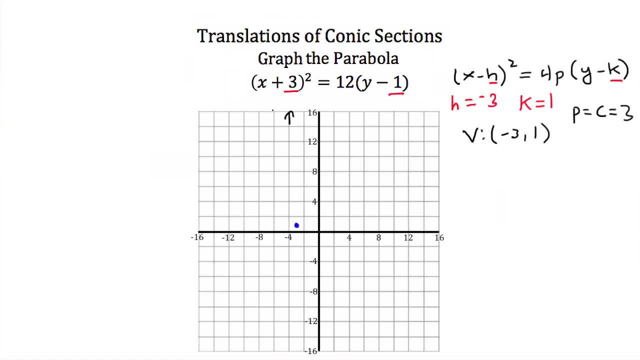 parabola is going to open in that direction. That means our focus is going to be above our vertex and our directrix is going to be below. It also means that I'm going to have an axis of symmetry that passes through that vertex and our focus when we find it, And that axis of symmetry is going to 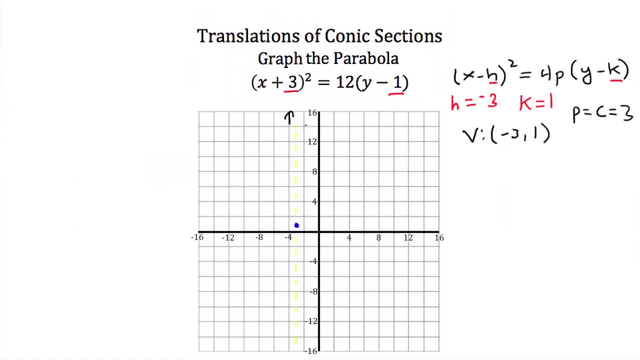 be parallel to the y axis, So our parabola will be symmetrical across this axis, and this axis is the line. x is equal to negative 3.. Now our p, p or our c value, that's equal to 3, and that means that our focus is going to be. 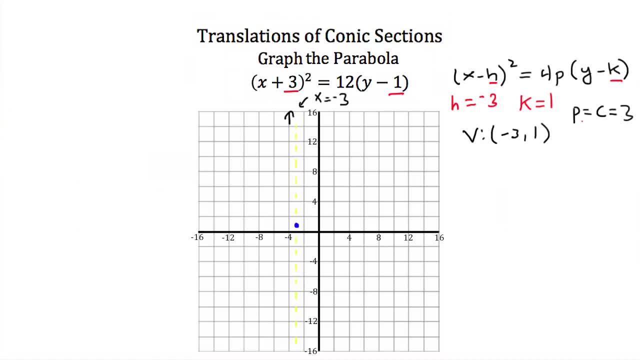 3 units above our vertex or along our axis of symmetry. so if I'm starting at negative 3- 1 and I move upward 3 points, I'll find out that my focus is the point negative 3- 4. if I go back to my vertex and I go down 3 units, I should run into 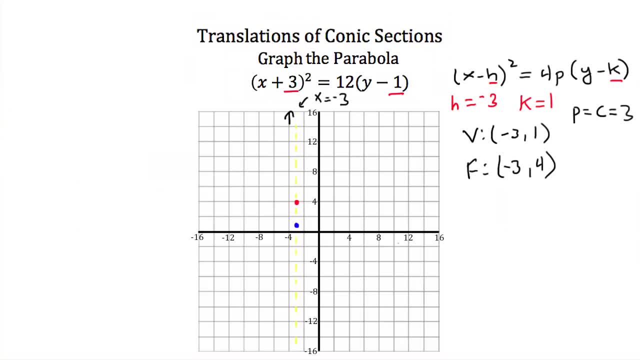 my directrix, which is the line perpendicular to our axis of symmetry. that means my directrix would be: the line y is equal to negative 2. so I found all the important characteristics of my parabola and now I just need to sketch it and this parabola should look like. 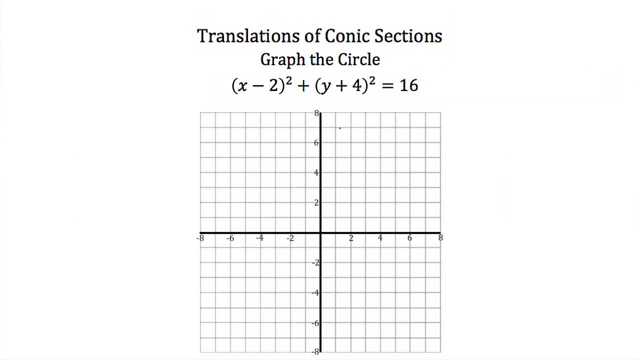 something like this: so now let's try graphing this translated circle. here we have the equation x minus 2, squared plus y plus 4, squared is equal to 16. this is in the standard form of x minus h squared plus y minus k, squared is equal. 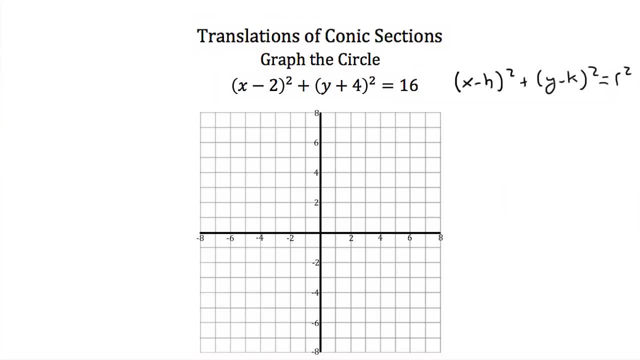 to R squared again. right away, we can tell that our H is 2 and our K is a negative 3, and that's what we're going to do next. we're going to take our negative 4. so immediately we've found the center of our circle. it's the point. 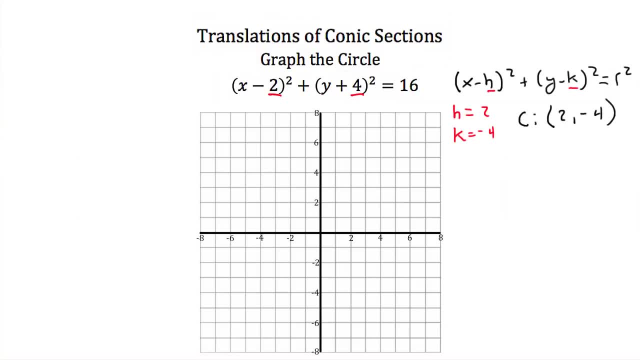 2 negative 4. we also know that 16 is equal to R squared. R squared is equal to 16. take the square root of both sides and you'll find out that R is equal to positive or negative 4, but R is a distance, so we don't worry about the. 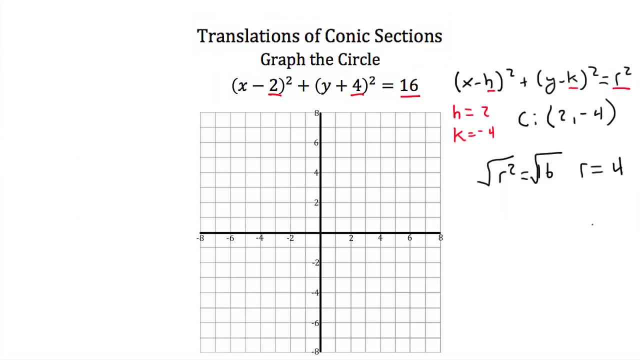 negative version. we just say that R is equal to 4. now we have all the information we need to know about our circle, so let's go ahead and start our calculation. we need to graph this circle. we have the center 2 negative 4. now every point on this circle is a radius of 4 away, or a distance of 4 away the 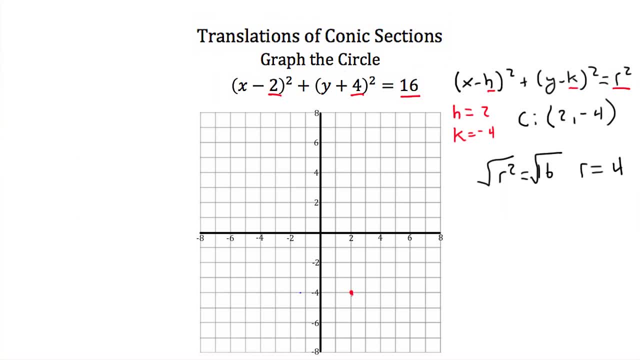 easiest points to find are the ones that are horizontally or vertically a distance of 4 away from this center. so if I'm at 2 negative 4 and I go to the right 4 units, I'll end up at 6 negative 4 if I go. 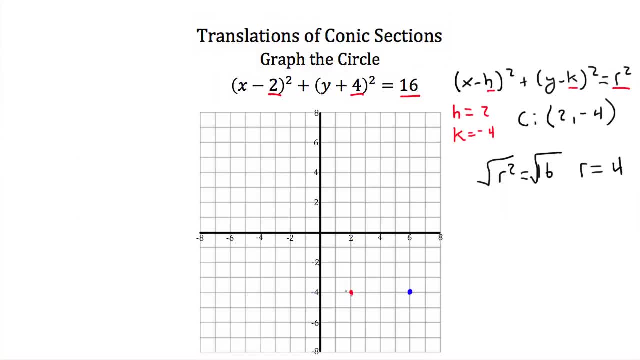 back to my Center- 2 negative 4, and I go to the left, our units or 4 units, I'll be at the point negative 2 negative 4. if I go back to my center again and I go up four units, I'll be at the point 2: 0 and then if I go back to my center and go 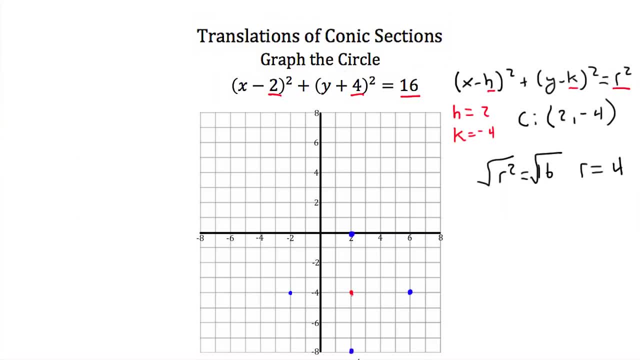 down four units, I'll be at the point 2 negative 8 connect the dots with our circle, and that would be the graph of x minus 2 squared plus 1. y plus 4 squared is equal to 16.. Now let's try graphing a translated ellipse. Here we have the 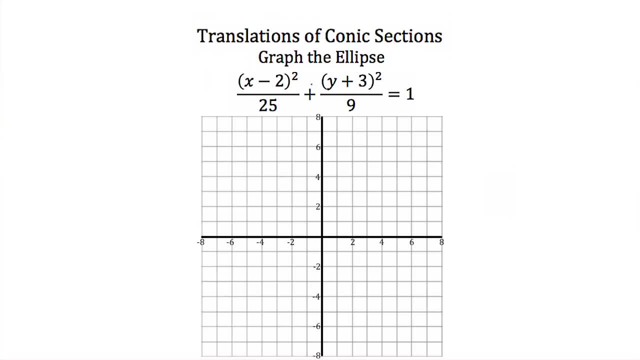 equation: x minus 2 squared over 25, plus y plus 3 squared over 9, is equal to 1.. This is in the standard form: x minus h squared over a, squared plus y minus k squared over b squared, is all equal to 1.. Again, just looking at these equations, we can tell that our h value is 2 and our k value is. 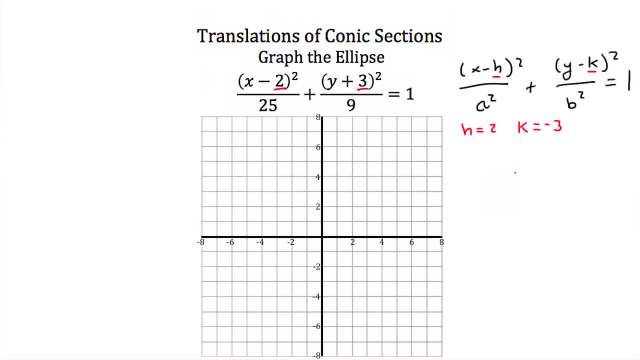 negative 3.. So we found the center of our ellipse. it's the point 2 negative 3.. I can plot that point. it's right there. Now, looking at this equation, our a squared value is 25 and our b squared value is 9.. 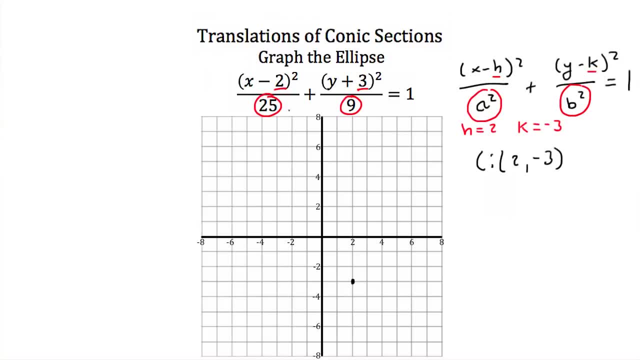 If you were to take the square root of both of these numbers, you'd find out that a is equal to 5 and b is equal to 3.. My a value is larger, which means my major axis of symmetry is going to be parallel to the x-axis. It always passes through the center. 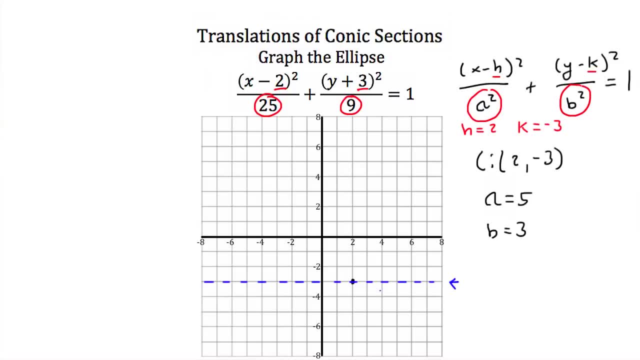 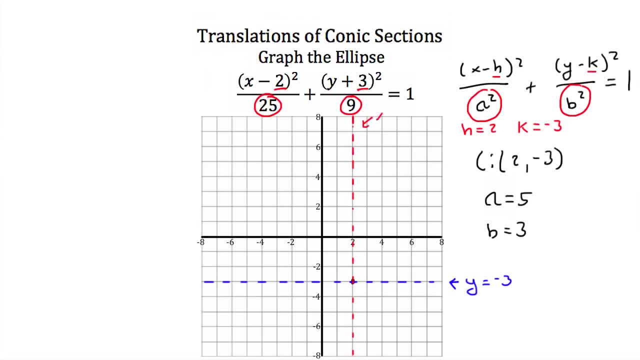 x is equal to 2.. Now if we start at this center and I go a distance along my major axis, so a distance of 5, then I'll come to the point 7, negative 3.. If I go a distance of 5 to the left, I'll come to the point negative 3, negative 3.. If I go a b distance, 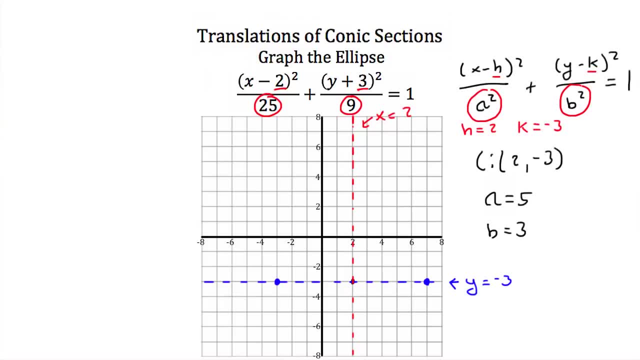 along my minor axis or in the y direction from my center. well, I'm starting at 2 negative 3, so I go up 3 and I'll be at the point 2: 0.. If I go back to my center and I go down 3 units, I'll be at the point. 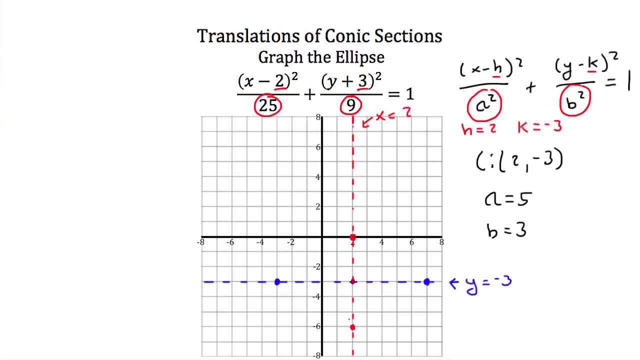 2 negative 6.. So by using my a and b values, I've just found that I've got a distance of 5 to the left. So I'm going to go down to all four of my vertices If I want to find my c values. well, my foci are going to be on my major axis, and that's the x direction, or parallel to the x axis. 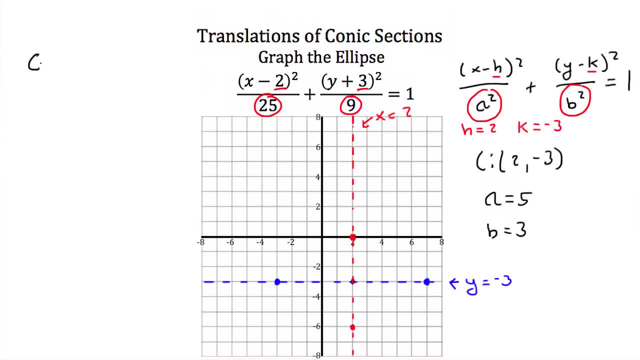 So I would use the equation: c squared is equal to a squared minus b squared. My a is 5, my b is 3, so c squared is equal to 5 squared minus 3 squared. So c squared is equal to 25 minus 9, or c squared is equal to 16, and that means c is equal to 4.. 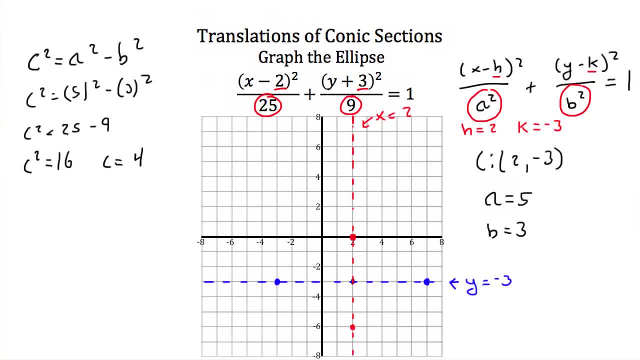 So my foci are a distance of 4 units away from my center along my major axis, and my major axis is the line y is equal to negative 3.. So I go to my center and I go along this axis 4 units, and I'll find that one foci is the point 6, negative 3.. 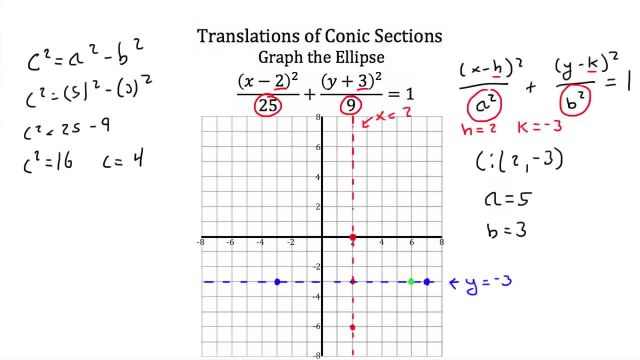 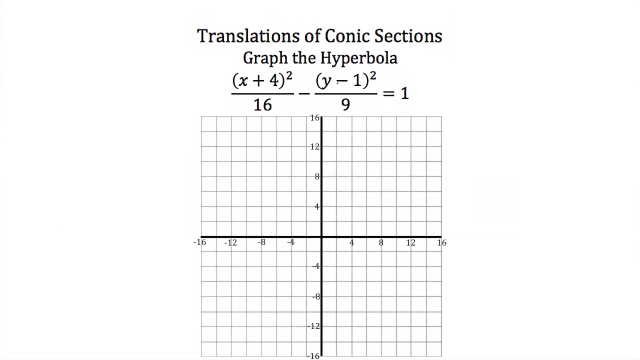 And the other one is negative: 2 negative 3.. So I found all my information for this ellipse and now I can graph it. My ellipse would look something like that Now, lastly, let's try graphing the hyperbola: x plus 4 squared over 16, minus y minus 1 squared over 9, is equal to 1.. 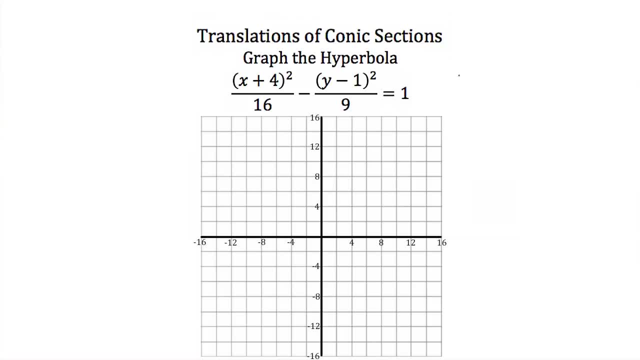 This equation is in the standard form for a hyperbola that's been translated or moved. That form is x minus h, squared over a squared, minus y minus k squared over b squared, and that's equal to 1.. Our y term is what's being subtracted, which means this hyperbola is going to open in the positive and negative x directions. 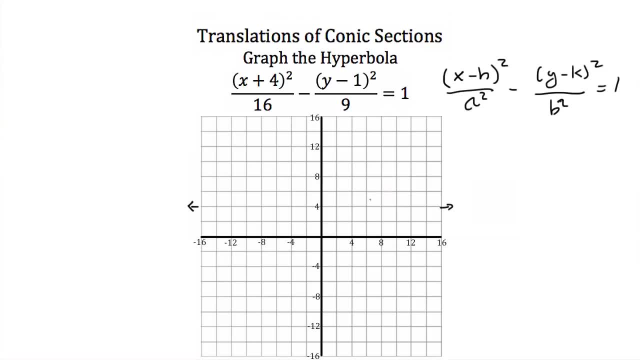 I can find the center of my hyperbola, because my h value is a negative, Negative 4 and my k value is a positive 1.. So that means my center is going to be the point negative 4, 1.. Now I also can find my a and b values. 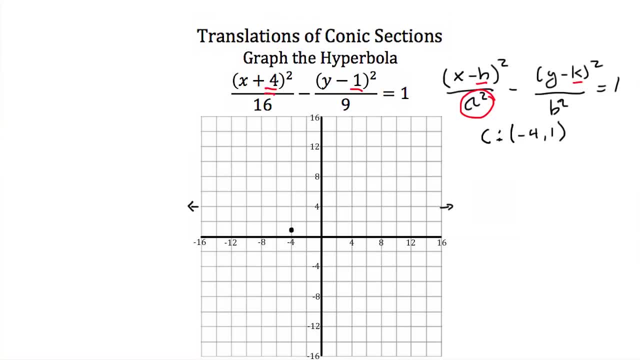 a squared is equal to 16 and b squared is equal to 9.. That means that a is going to be equal to 4 and b is going to be equal to 3.. Now my a is underneath my x variable, which means that's going to be the size of my axis of symmetry in the x direction. 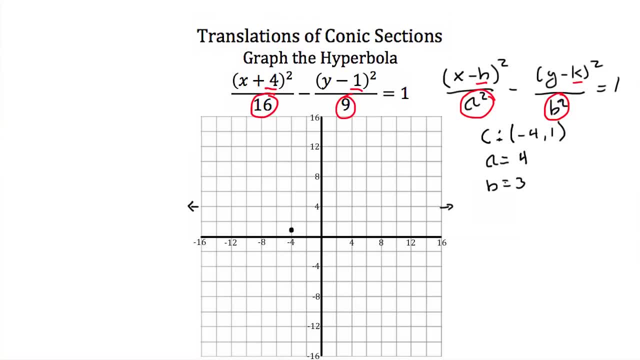 My b value is 3 and it's underneath my y variable, which means that's going to be the length of my axis of symmetry in the y direction. Now I have two axes of symmetry. They both pass through my center. If I'm going 4 in the x direction, then I start at my center and I move 4 units to the right. 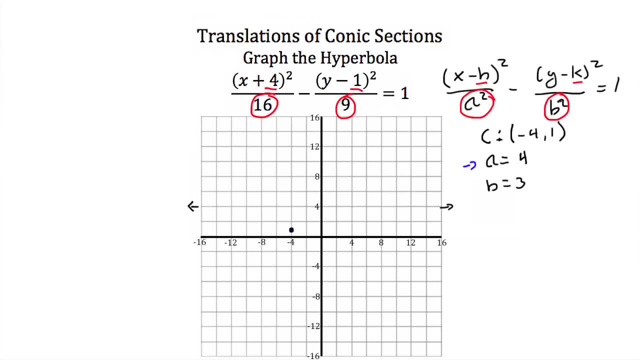 So if I'm at negative 4, 1, I'll end up at 0, 1.. If I go to the left, I'll end up at negative 8, 1.. Now for my b value. if I'm at my center of 1, negative 4 and I go up 3 units, I'll be at 4, negative 4.. 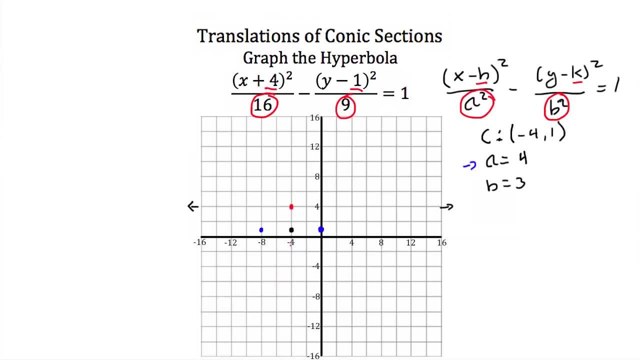 And if I go down 3 units I'll be at negative 4.. Now if I want to find my c values or the location of my foci, I just use the equation: c squared is equal to a squared plus b squared. If we plug in 4 and 3 for a and b, we'll have 4 squared plus 3 squared. 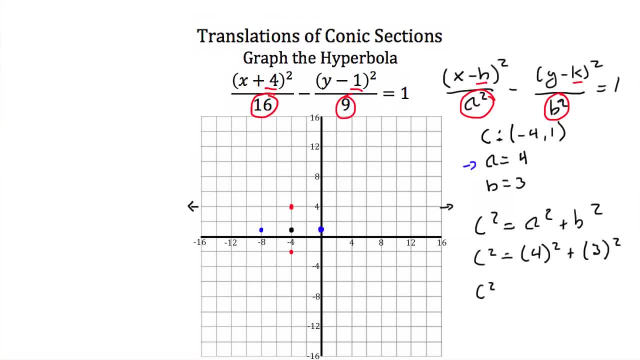 4 squared is 16, 3 squared is 9.. 16 plus 9 is 25.. So c is equal to 5.. Now my a value is larger than my b value, which means my transverse axis is going to be parallel to the x axis. 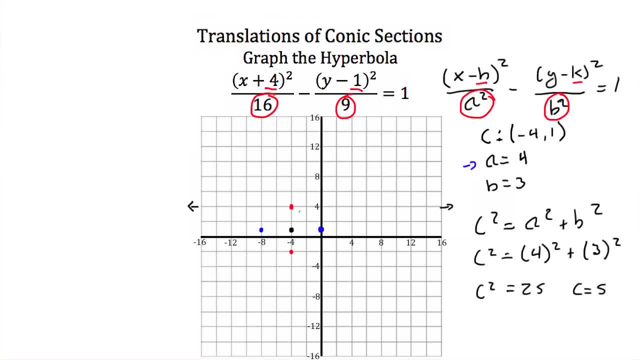 And my foci are a distance of 5 away from my center. So if I start at negative 4, 1 and I go 5 to the right, I'll be at 1, 1.. And if I go 5 to the left, I'll be at negative 9, 1.. 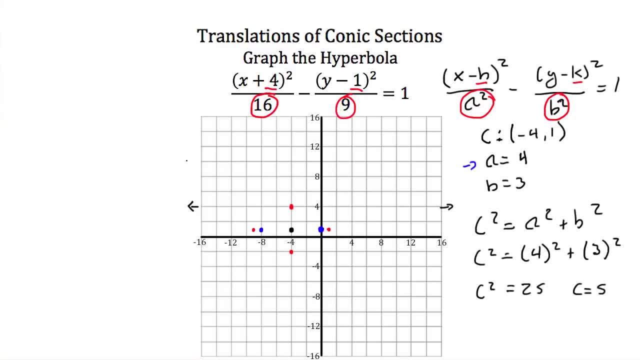 Now that I've found my foci, the last thing I have to do is find my asymptotes. I know my asymptotes pass through the center and they have the slope plus or minus b over a. Well, my b is 3 and my a is 4, so my asymptotes are going to have the slopes plus or minus 3 over 4.. 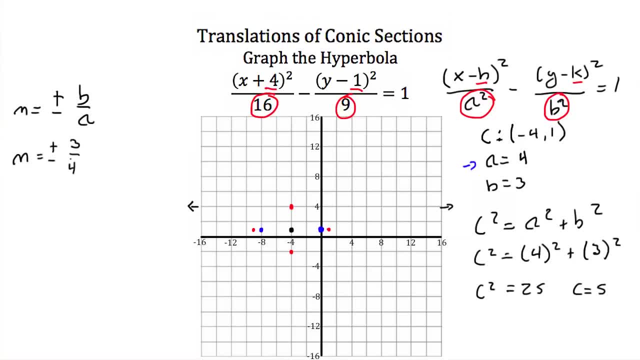 Plus or minus 3 rise over 4 run. So if I start at my center And I go up 3 and over 4. And I can connect that point to my center, I'll see that one of my asymptotes looks like that. 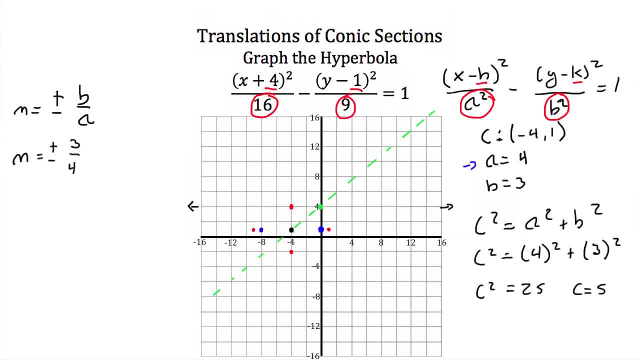 If I go back to my center- and this time I go down 3 and over 4. And I connect that point to my center- I can see my other asymptote is going to look like that. So I have my vertex, I have my asymptotes and I have my foci. 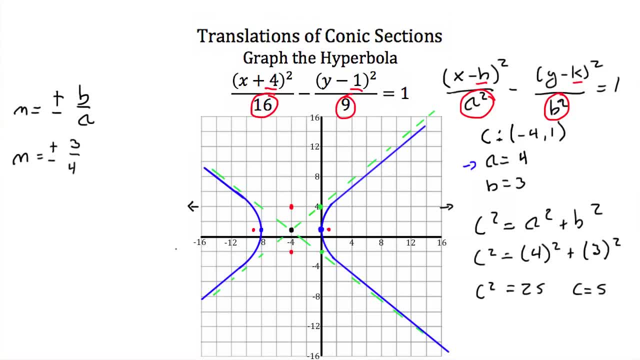 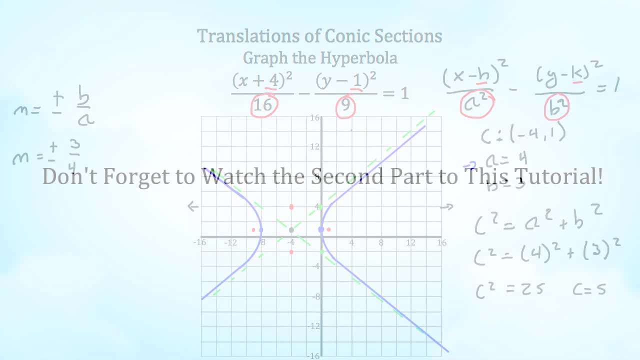 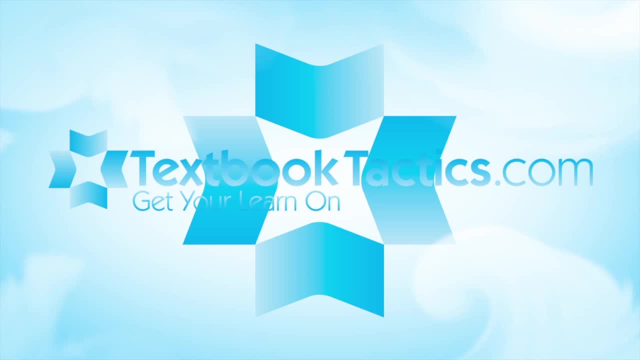 My hyperbola should look something like this, And that would be the graph of x plus 4 squared over 3.. Over 16 minus y minus 1 squared over 9 is equal to 1.. Thank you for watching.